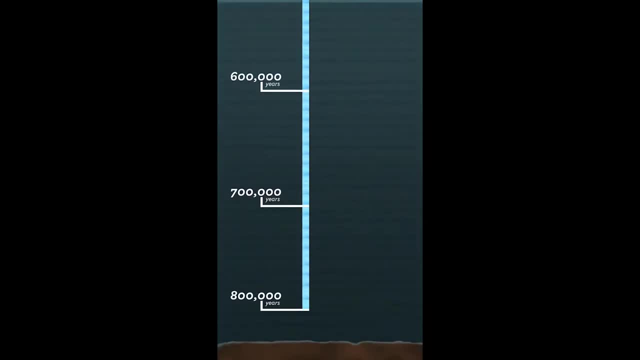 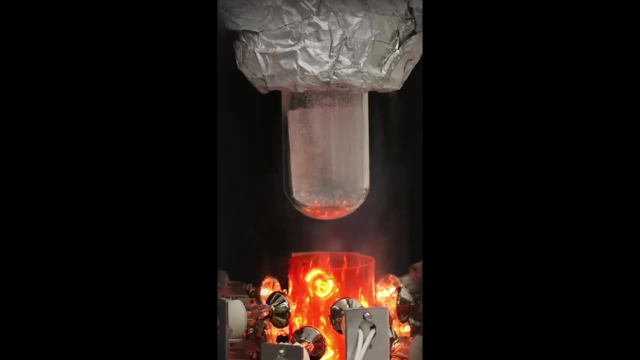 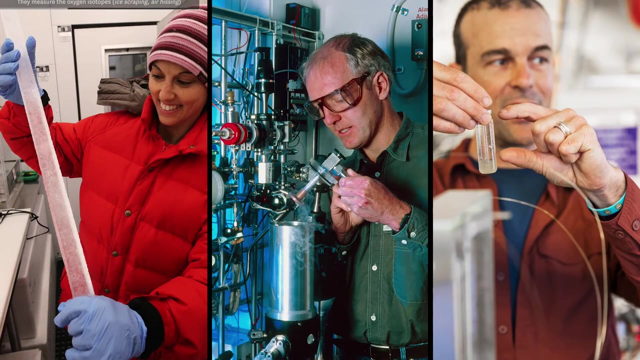 It preserved 800,000 years of information. In the laboratory, scientists melt samples of the ancient ice. They measure the oxygen isotopes to determine how cold it was when the snow fell. In burner-greased containers, slices of paper are put in tensions to test. They predict changes inleye long and heat™ limit, the particularly extreme continued activity. H startup is significantly adjusting global temperature as well. Its levels of Daily Whenaha have decreased by over 200 percent, as well as the levels of the observed globally ageing temperatures. 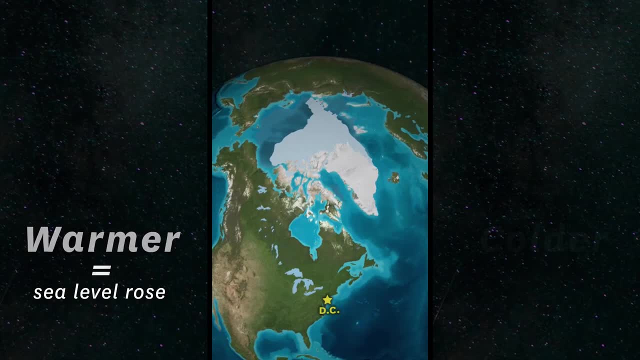 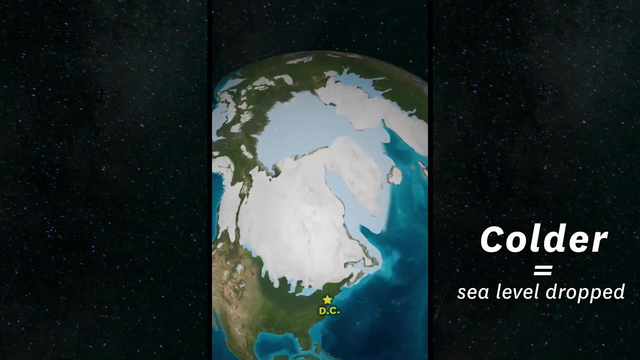 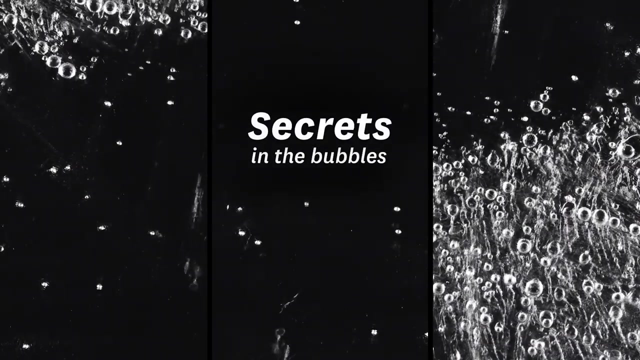 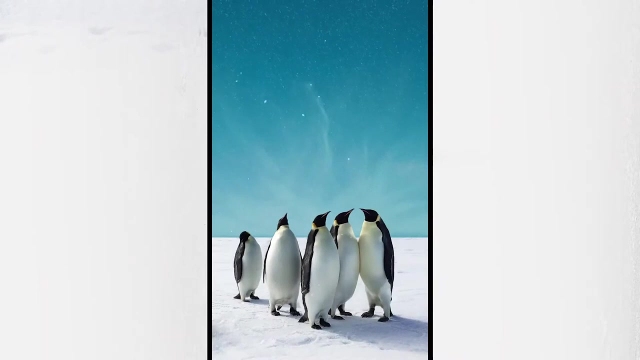 In smash-houses awards of different вещies such as stick, gamma light, etc. massive ice sheets spread Sea level, dropped as water froze into ice. Ice holds more secrets, Not just about past temperature, but about past atmosphere too. 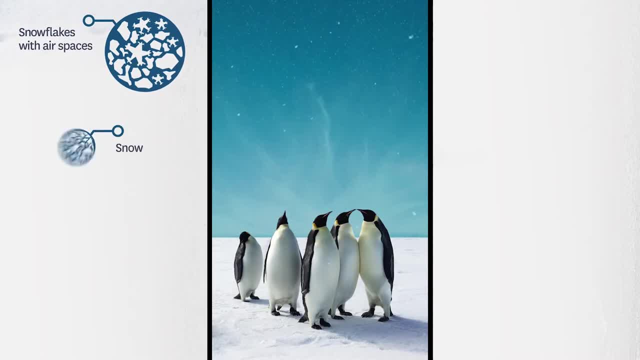 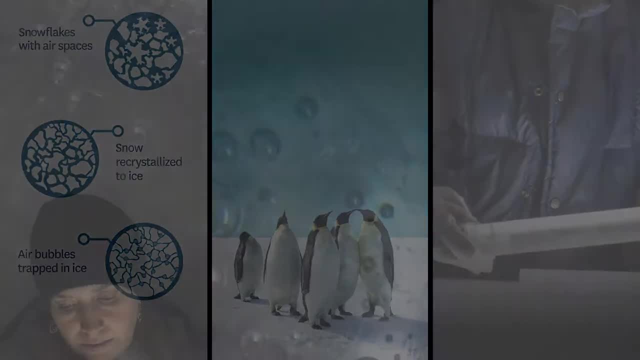 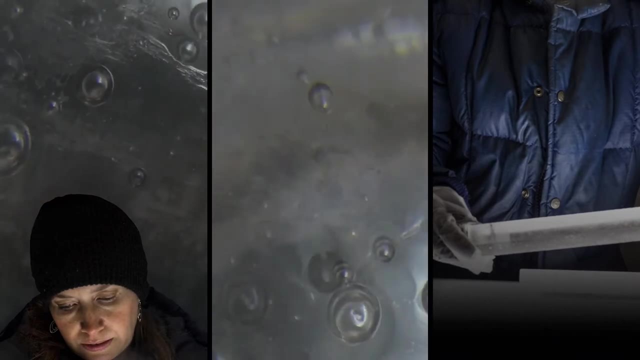 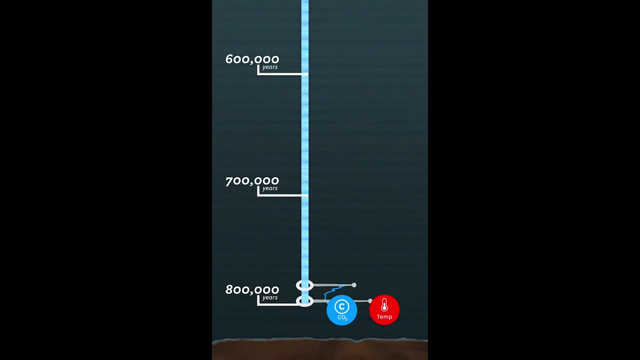 When snow falls, it traps air. That air is compressed into bubbles. as the snow compacts into ice In the lab, scientists can tap into the bubbles and measure their carbon dioxide levels. Decades of research revealed that changes in carbon dioxide are linked to changes in temperature. 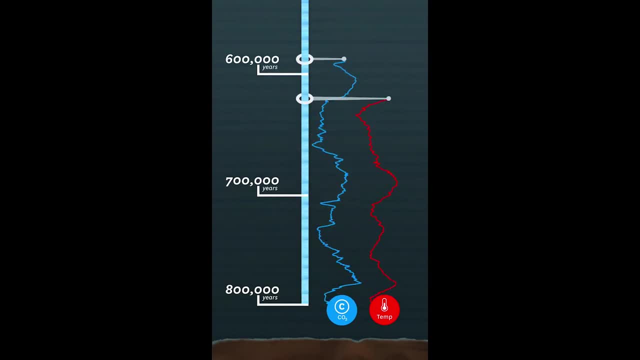 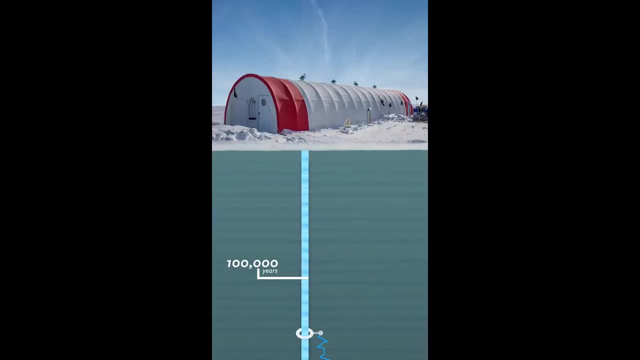 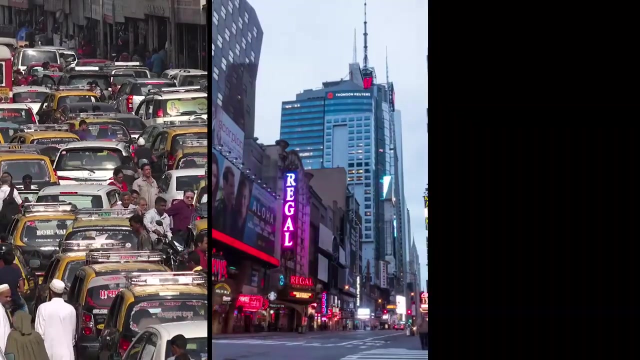 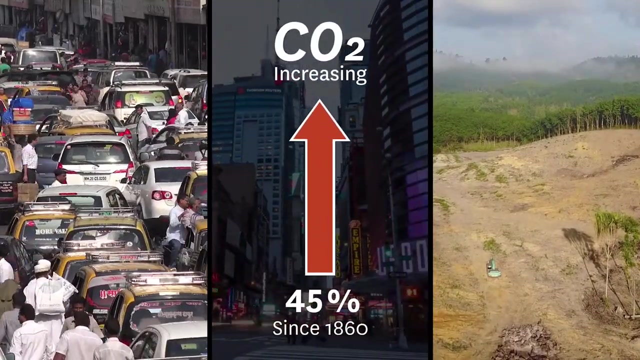 Look at these two graphs. When CO2 increased, temperature went up. When CO2 decreased, so did temperature. Today, CO2 is skyrocketing, higher than any time in the past 800,000 years, as we burn fossil fuels and cut down forests. 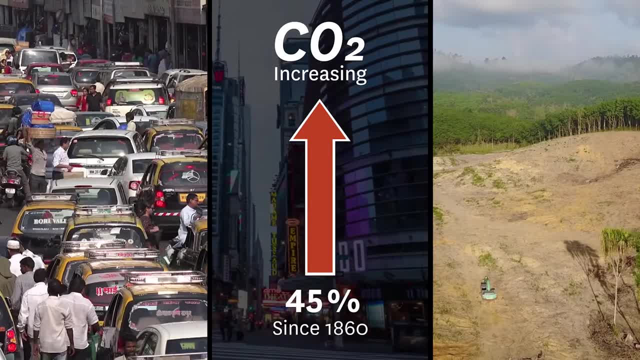 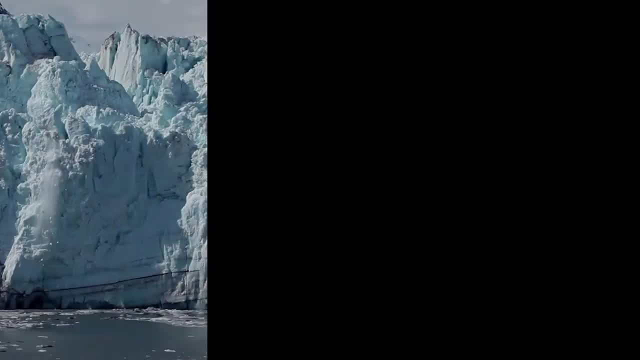 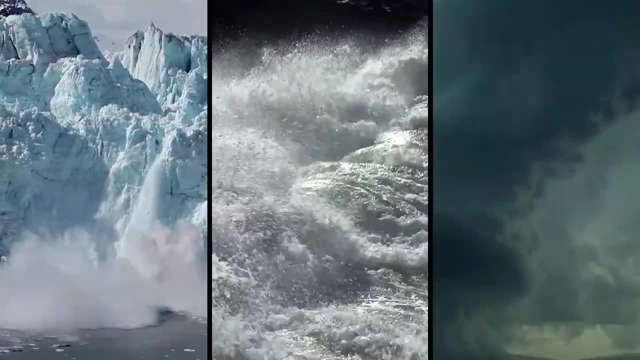 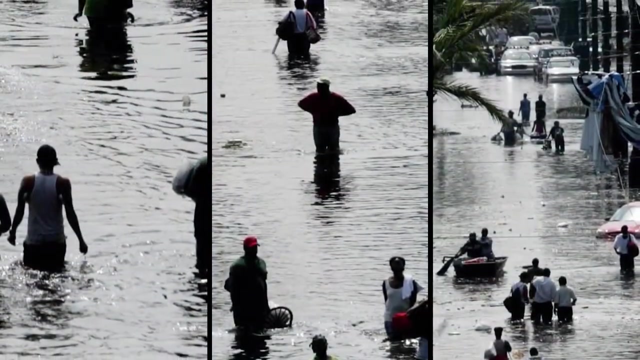 This time, humans are the reason Earth's temperature is rising. Just like in the past, the climate is responding to the increase in CO2.. Ice is melting, Sea level is rising And storms are becoming more powerful. These rapid changes in climate, 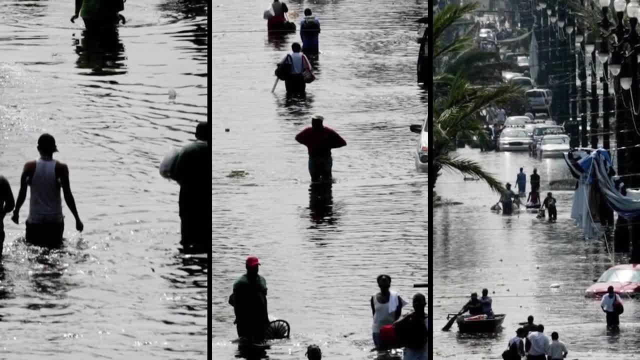 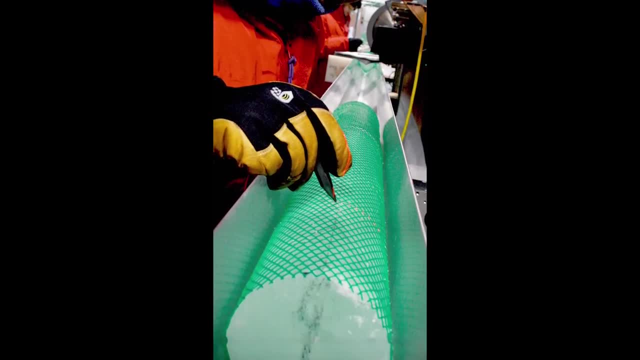 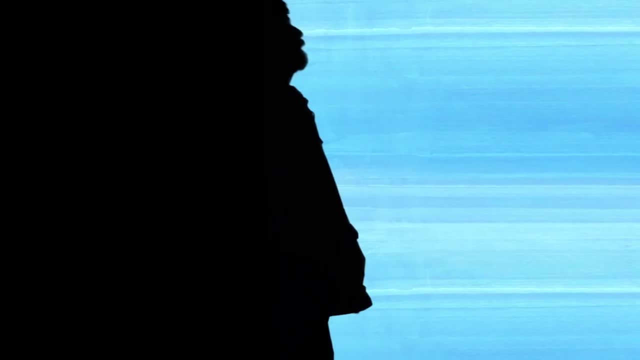 threaten human lives and profoundly impact all life on Earth. Knowing the story of Earth's climate, the Earth's climate past, can help us prepare for Earth's climate future. What we do now will write the next chapter in the ice.